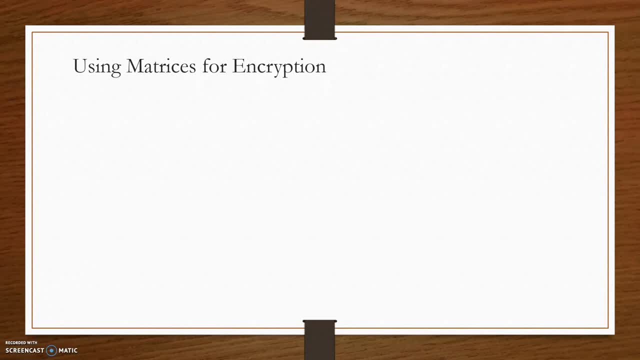 much larger matrices are typically used for this type of code. the bigger, the harder it is to unencrypt. First we need to figure out what the message we want to send is. Here we can just have our message: be Meet Tomorrow at Midnight- a real creepy message. 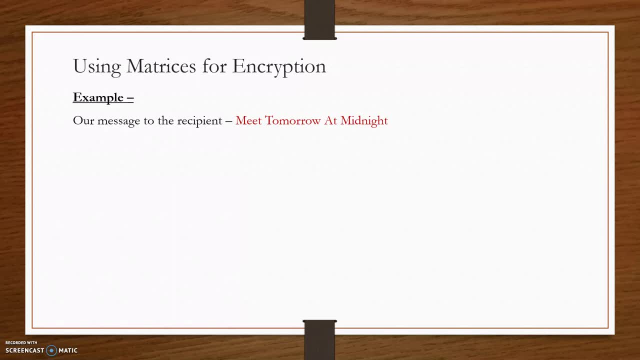 to somebody that doesn't know what it is. Next we will set our encoding matrix and also our decoding matrix. The recipient will need to know at least one of these matrices so they can find the inverse by row-reducing. whichever matrix you want. 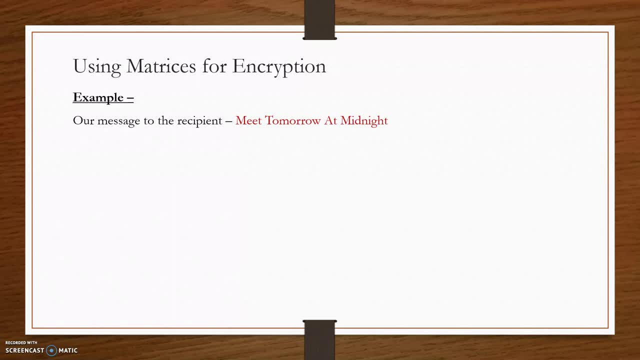 Next we need to tell them, augmented with the identity matrix, to find the other matrix to either read or send out more messages. Here are the matrices we will use for our example. Now we will assign each letter of the alphabet a number, in order. 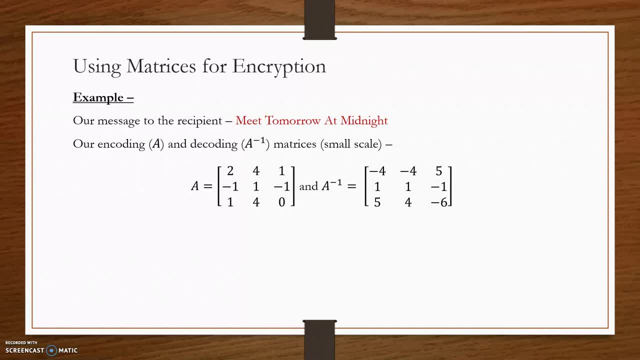 For example, A would be equal to 1,, B would be equal to 2, and so on. A space or a break will be assigned the number 27,, because there's only 26 letters in the alphabet. Now we translate our message into these numbers, as you see below. 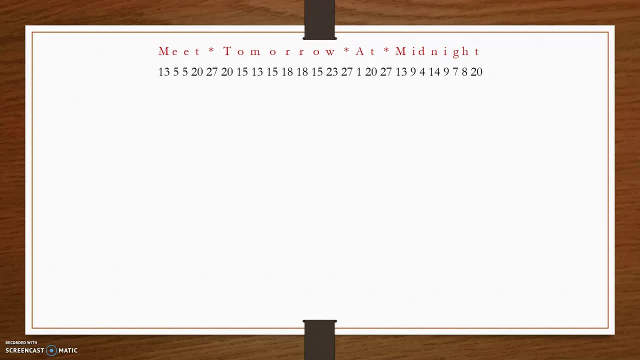 Now that we have our translated code, we need to put these numbers into vectors. Since we are using a 3x3 matrix, we break the enumerated message above into a sequence of 3x1 vectors, like so. Note that it was necessary to add two spaces, or 27s, at the end of the message to complete. 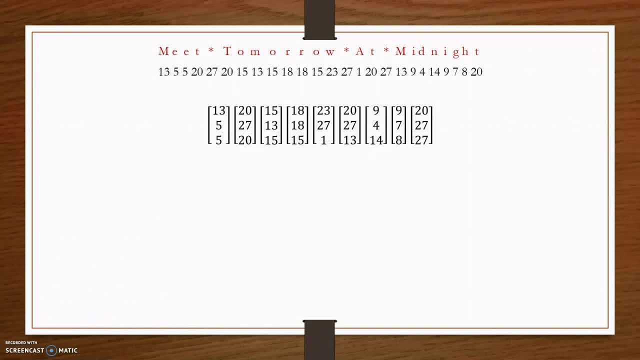 the last vector. We now encode the matrix by multiplying each of the above vectors, Okay, by the encoding matrix. This can be done by writing the above vectors as columns of a matrix and then perform matrix multiplication of that matrix with the encoding matrix, like so. 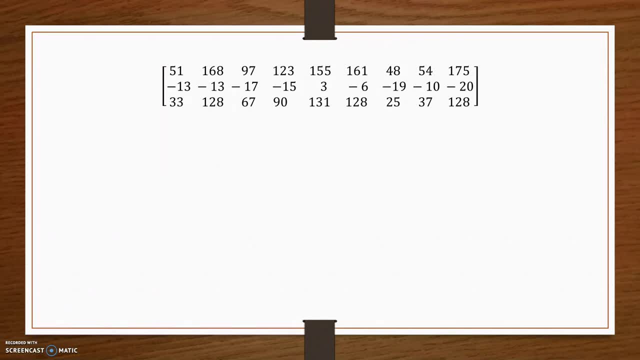 The columns of this matrix give the encoded message. The message is then transmitted in the following linear form: To decode the message, the receiver writes this string as a sequence of 3x1 column matrices and repeats the technique using the inverse of the encoding matrix. 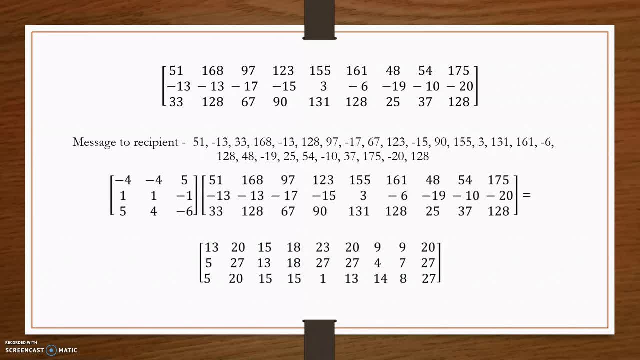 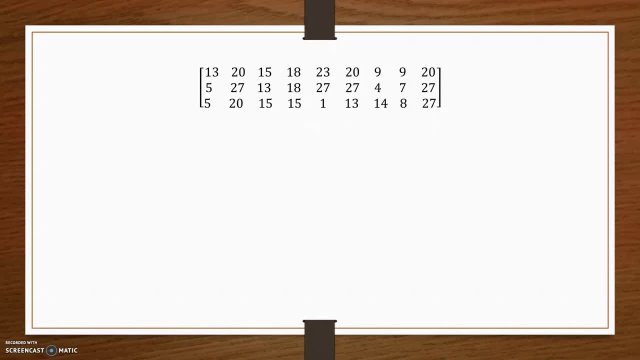 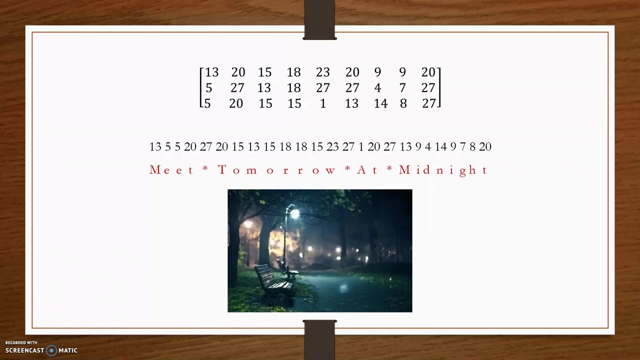 Thus to decode the message. they will perform the matrix multiplication and receive a matrix that should look familiar to you. The columns of this matrix, written in a linear form, give the original message, And now you can meet in secret with confidence that no outsiders to your conversation will. ever be aware.